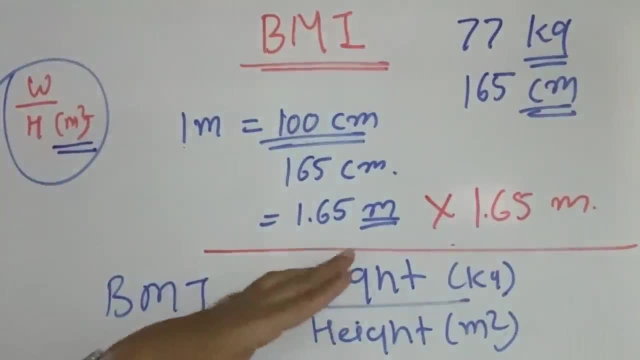 simple. Okay, So I use the formula here. What do we have? So we have 1.65 meters in the meter, which we have to double multiply. So how will we use this in the formula? We have to write the formula here in which the weight is divided by the height in the meter. 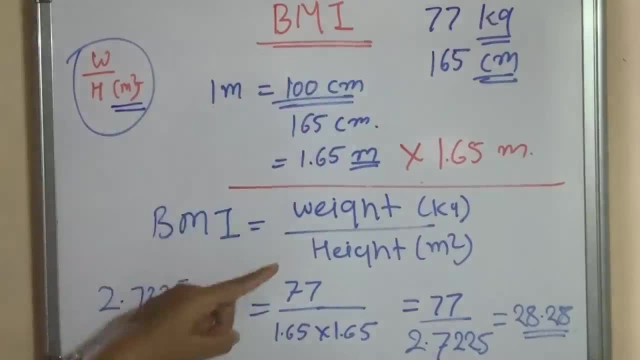 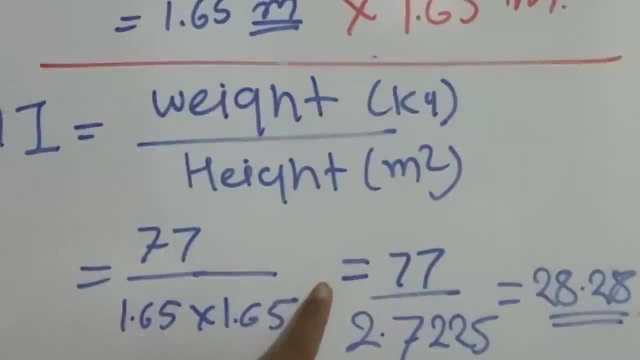 square. So the weight we took here is 77 kg and the height is 1.65, which we converted into centimeters in the meter, and multiply it by again 1.65 meters, because we are taking out the square. After that our equation of multiplication will be 2.7225.. When we divide, 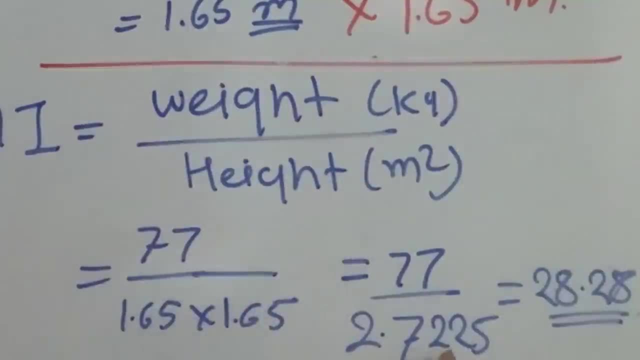 77 divided by 2.7225, the value will come, that is, 28.28.. Now we will see what is the reading of 28.28.. How will we understand it? Fat percentage is equal to 1.65 meters, So we have to write. 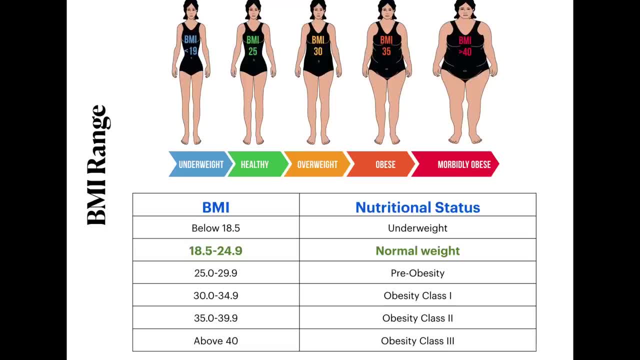 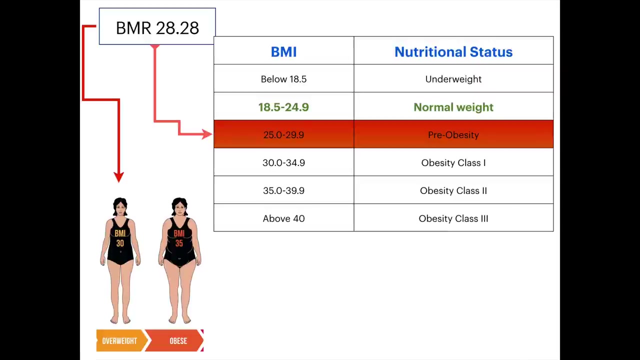 the figure of β. So what is the fat percentage of this bandha? Here the reference range of BMI of WHO is given like this, as you can see in the table, And the normal weight range here is 18.5 to 24.9.. According to the example we calculated, 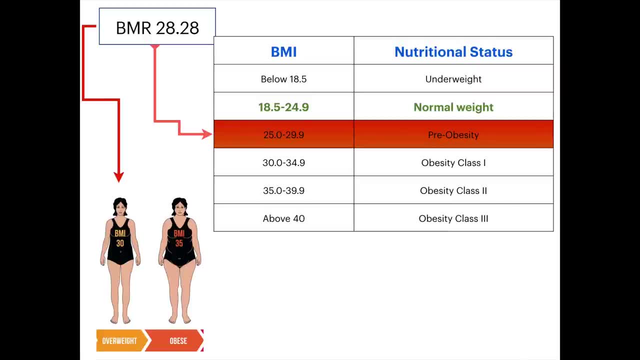 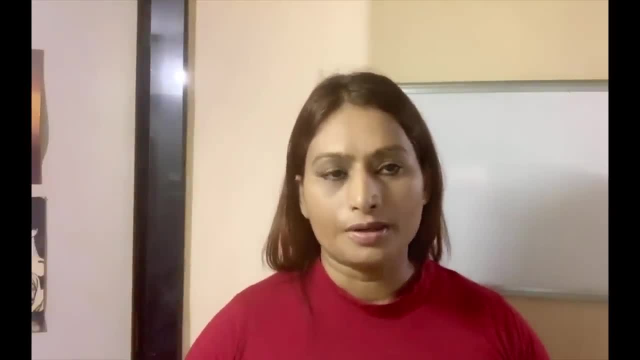 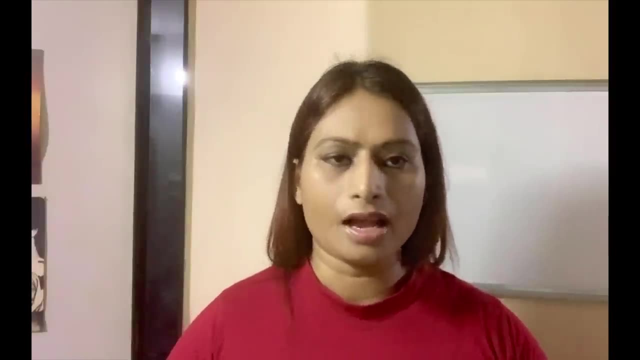 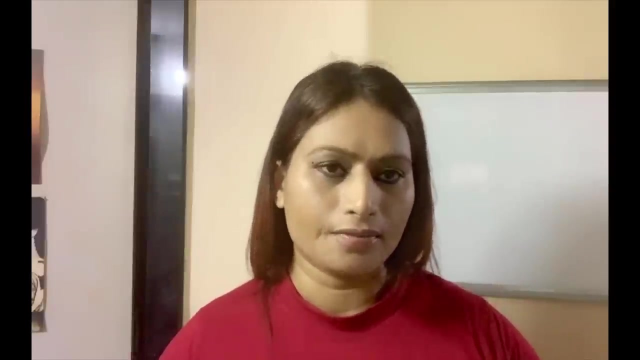 28.28 is the range that indicates the Pre-Obesity Stage. So here we have seen how BMI is calculated and what are the things we need for BMI calculation. What does BMI interpret? How does it indicate our fat percentage? So all these things are very helpful to identify our fat percentage. 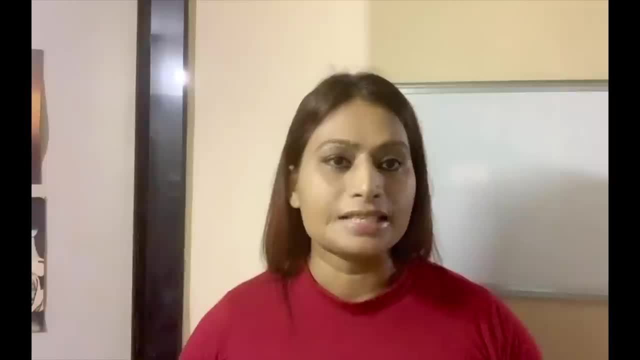 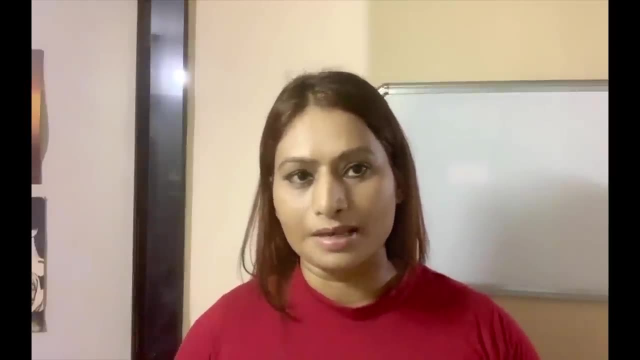 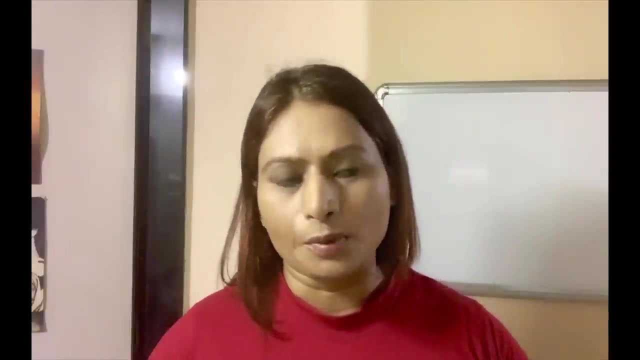 BMI is not a universally justifiable process to measure fat, So we can consider BMI as a basic level of measurement. Apart from this, you must have heard of hip-waist ratio, which is called apple shape and pear shape in fat profile. 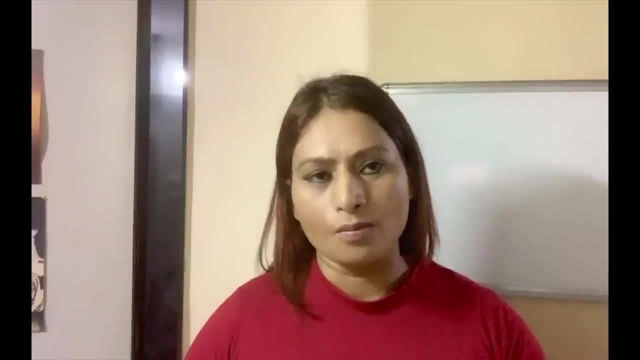 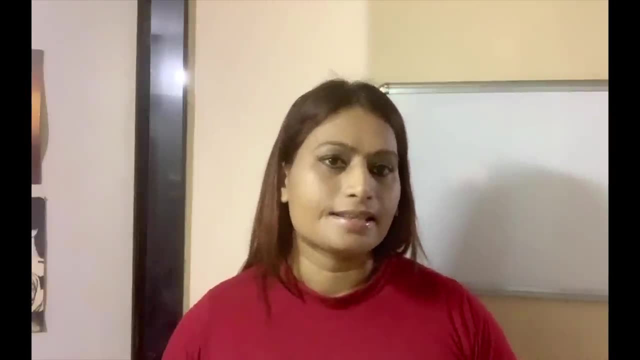 So waist-hip ratio is a very good technique of fat measurement, which I will explain in my next video. How can we measure WHR?